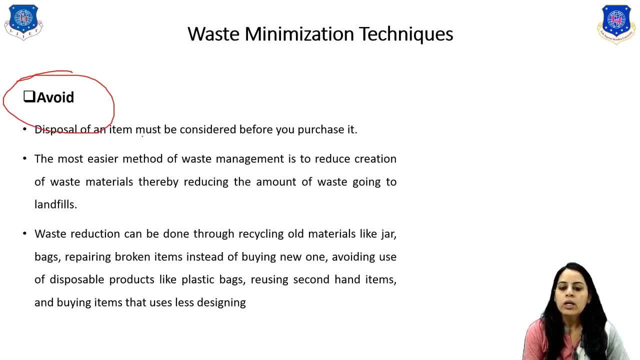 responsibility of the waste. Okay, Now we will start with the first one, which is avoid- okay so, the disposal of an item that must be considered before you purchase, right? So the most easier manner of the waste management is to reduce creation of the waste, waste management, thenриuse Radical waste. 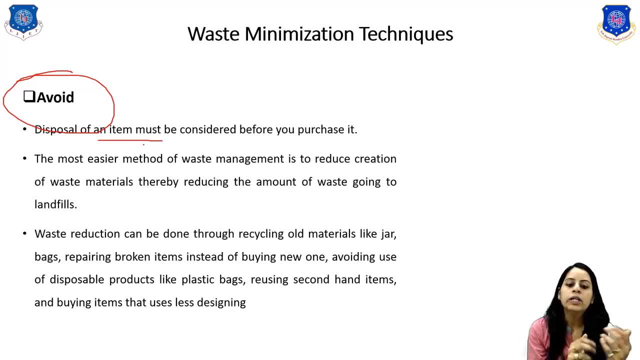 recycle- Okay- waste material, thereby reducing the amount of waste which is going to landfill, okay. so the waste reduction it can be done through the recycling of the old material, like a jar bag, repairing broken items that instead of buying a new one, avoiding the use of disposable product. 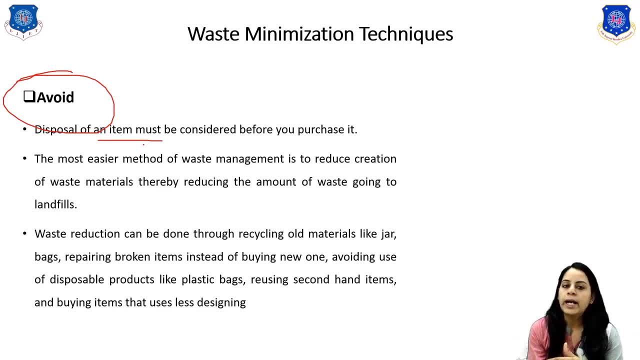 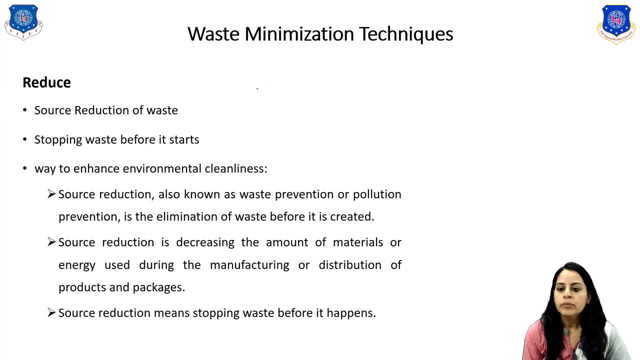 like a plastic bag. then reusing the second hand items: okay. then buying the item that use this design: okay. it means that the avoid: okay. the next one, which is the reduce. it means that the reduction in the source of the waste, okay. so the source reduction of the waste by stopping. 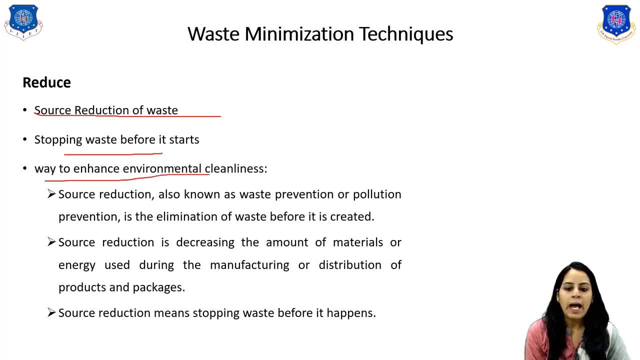 the waste before it's stuck right. so the way to enhance the environmental cleanliness, the first one, which is the source reduction, also know as a waste prevention or a pollution prevention, is the elimination of waste before it is created. okay, so the source reduction is reducing the amount of material or energy used during the manufacturing or distribution of. 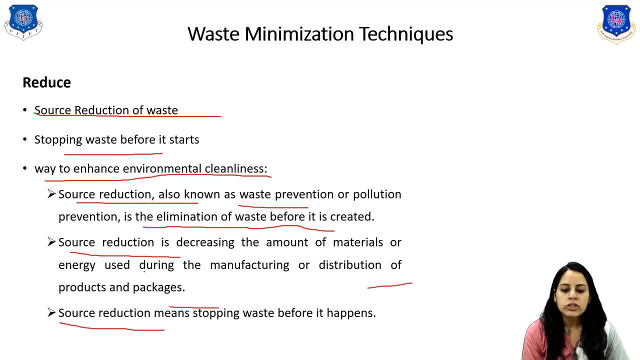 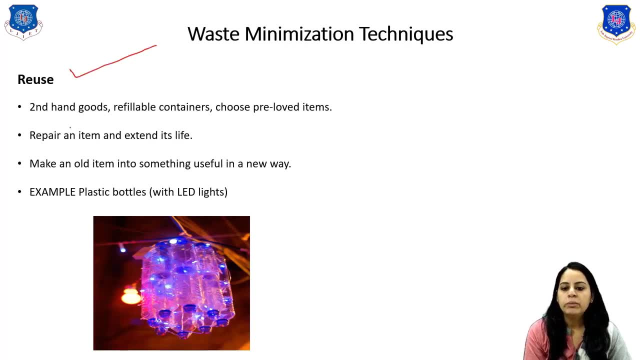 product and the packages, okay. the source reduction means stopping the waste before it happen, right. the next one, which is the reuse: it means that it is a second hand goods than a refillable container. then choose a free, low items, right. so the repair an item and extend its life. make an old item into 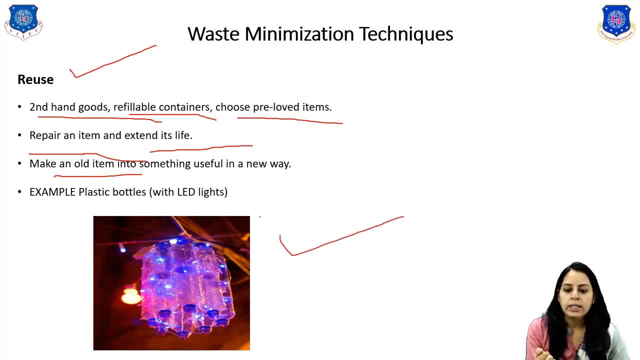 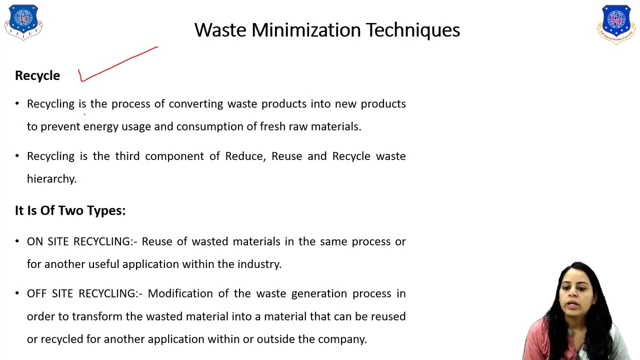 new one. so this is something useful in a new way. here you can see that the example are given. the example which is plastic vertex bottle which is reusable with the allowed likes right. so here the picture. you can see that now. next one which is a recycle: okay. 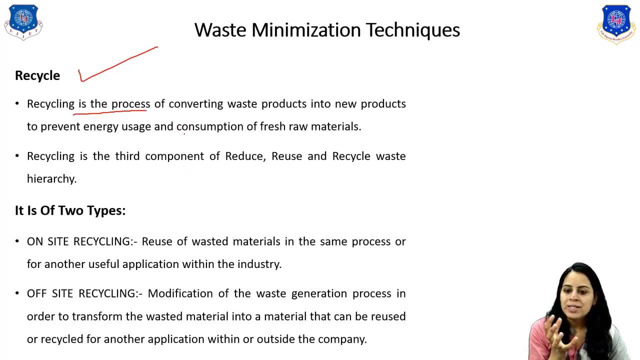 so the recycling is the process of converting the paste into the new product. it means that existing one which is replaced with the new one to prevent the energy uses and Ripasses and the consumption of Яй competition of the old one to high and low level product in the belki. 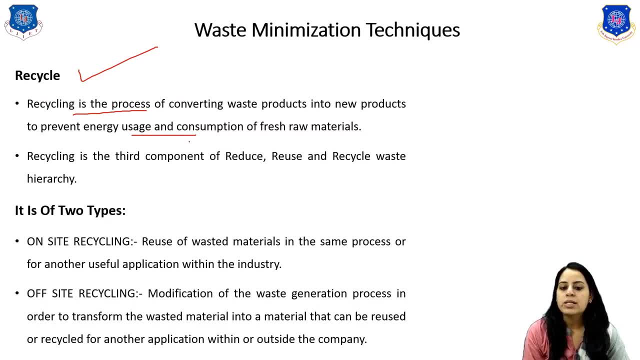 meny비section to prevent the energy uses and consumption of the new one in the previous process, in the next process. that recycling is done, so recycling is important. that recycling means aggressively, so recycling is done to α kg t so hard q Ortho夠, of the fresh raw materials. It is the third component of the reuse and recycle waste hierarchy. 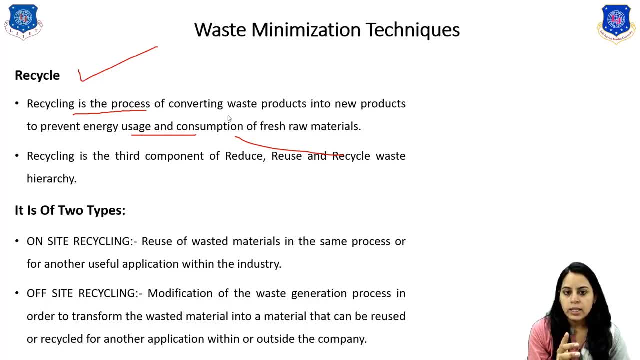 So the idea behind the recycling is to reduce the energy usage and reduce the volume of the landfill, reduce the air and water pollution, then reduce the greenhouse gas emission and the preserve the natural resource for the future. Now the recycling. it has two types. 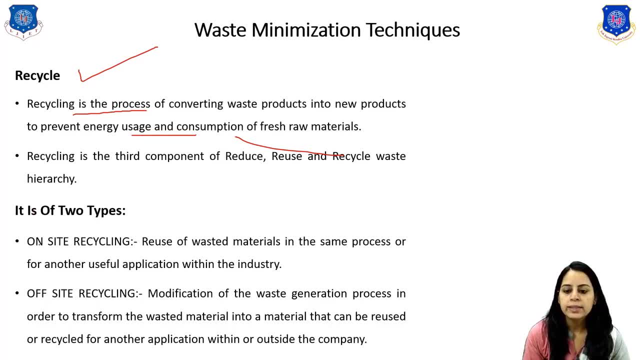 The first one, which is the on-site recycling, and the second one, which is the off-site recycling, So the reuse of the wasted material in the same process or for the another useful application within the industry. It means that on-site recycling, Because the material or the waste 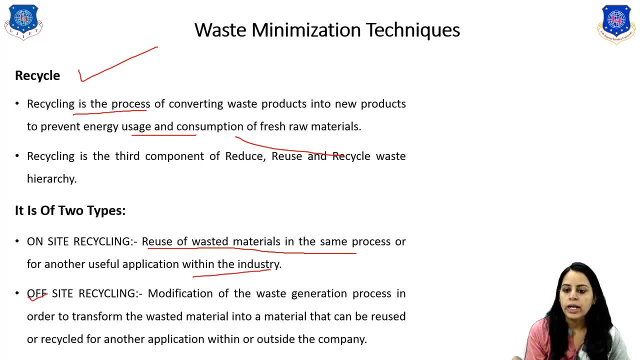 are useful in the industry. they are used in the industry. They are used in the industry, in the same industry. Then, off-site recycling: it means that modification of waste generation process in order to transform the wasted material into the material that can be reused or recycled. 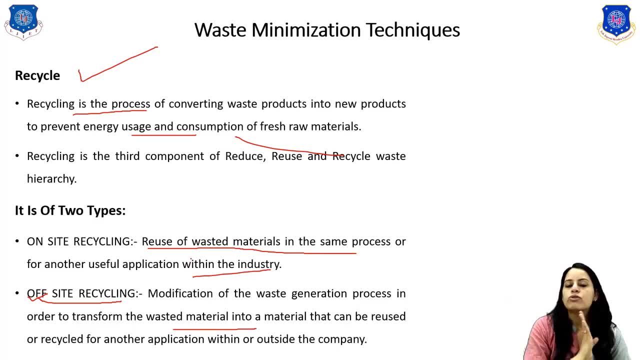 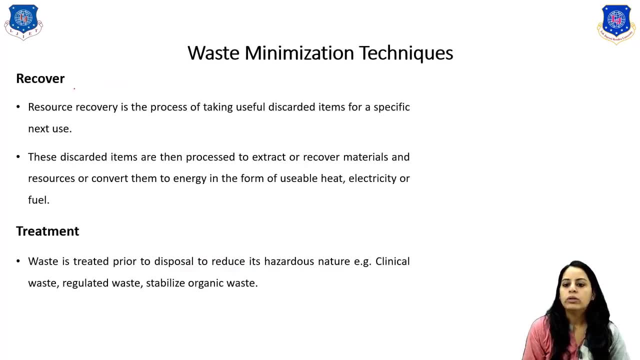 for another application, within or outside the company. This is a modification of the waste. Now the next one, which is the recover. So the resource recovery is the process of recycling or recycling of waste. So the resource recovery is the process of recycling or recycling of waste. 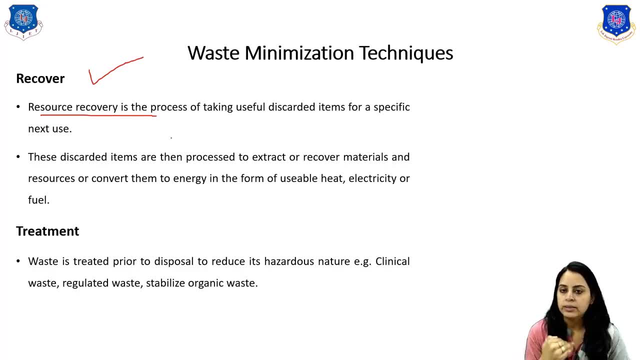 So the resource recovery is the process of recycling or recycling of waste. Taken the discarded item for a specific next use, So this discarded item are then proceed to extract or recover the material and resource, to convert them into the energy in form of the usable bit electricity or bit Recover. it means that resource to the waste, to the resource Recover. 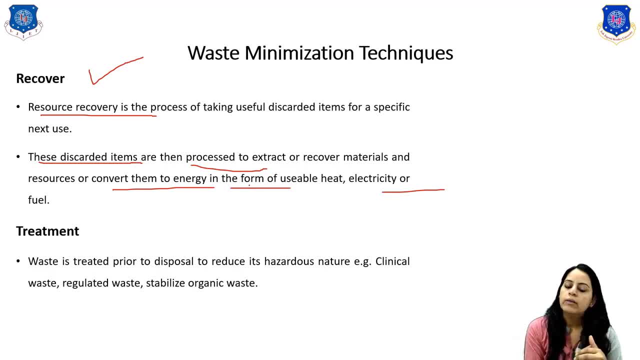 it means that the waste which is converted into the used waste in other ways, which is, which is converted into the resources, right. the next one, which is the treatment: okay, so the waste is treated prior to dispose, disposal, to reduce the hazardous nature, clinical waste, then regulated waste or stabilize the organic waste it means are treated. okay, there are lots of detailed treatment. 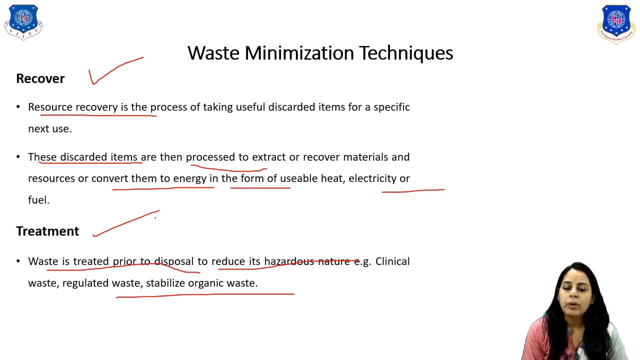 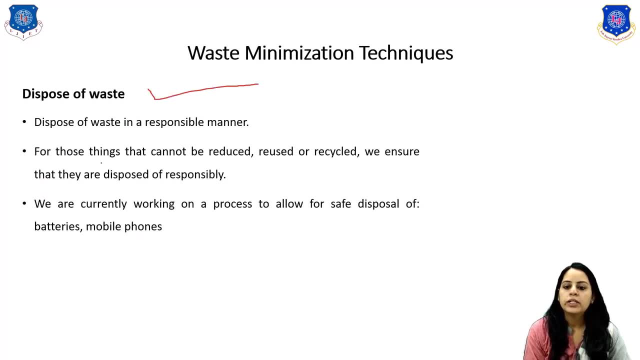 treatment for the waste: physical treatment and chemical treatment, okay, organic treatment and etc. now the last one, which is the dispose of waste. it means that it is a for those thing that cannot be reduced, reuse or recycle. so we ensure that they are dispose of the responsibility right, so we are. 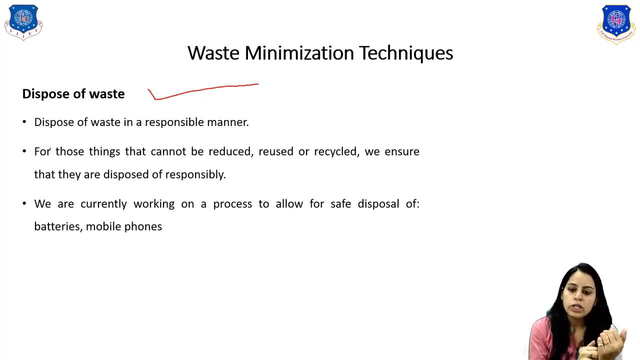 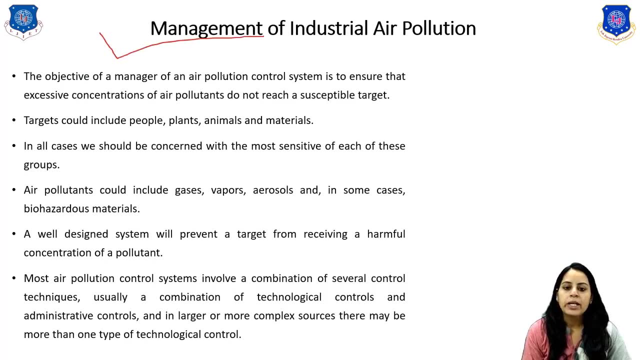 currently working on a process to allow for a safe disposal of the batteries and mobile phones and etc. okay, now the next one, which is the management of the industrial air pollution. okay, so this topic, which is the industrial air pollution management system, so the best. the first one. 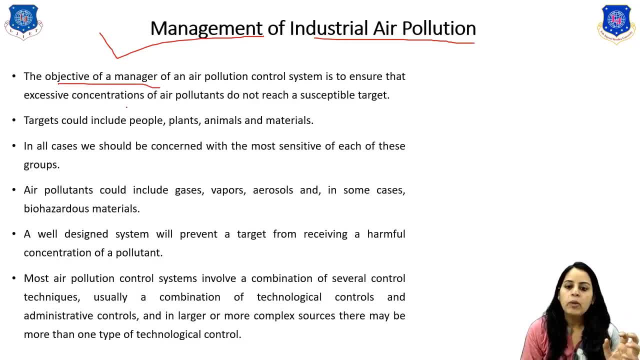 which is the objecting. okay, which is an air pollution manager of the non-pollution control system, is to ensure that excessive concentration of air pollution, air pollutant, do not reach a susceptible target. okay, susceptible target, so the target could include the people, plant, animals and. 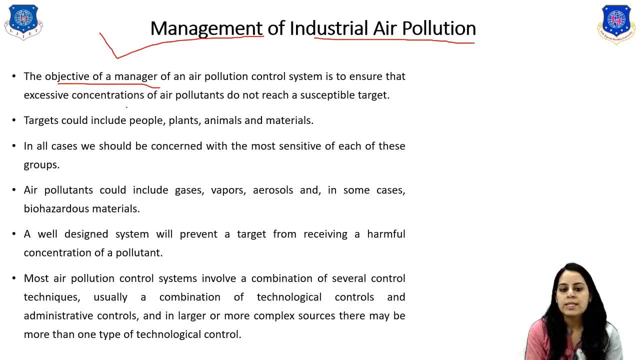 okay, so in our gas we should concern with the most sensitive of each of this group. so the air pollutant could include the gases, vapor, aerosol and, in the some cases of our hazard material. okay, so a well-designed system will prevent the target from receiving a harmful concentration of the. 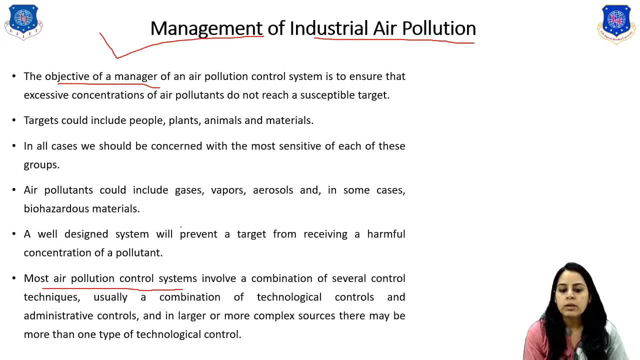 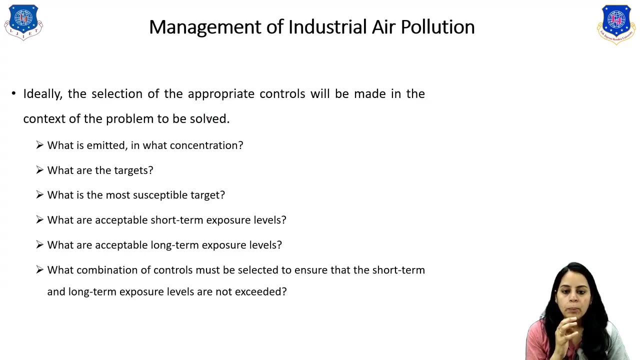 pollutant and the most are pollution. control system involve the company combination of the several control technique, usually combination of technological control and the administrative control and the large or more complex sources. there may be more than one type of the technological control. okay, now the ideally, the selection of of the across. 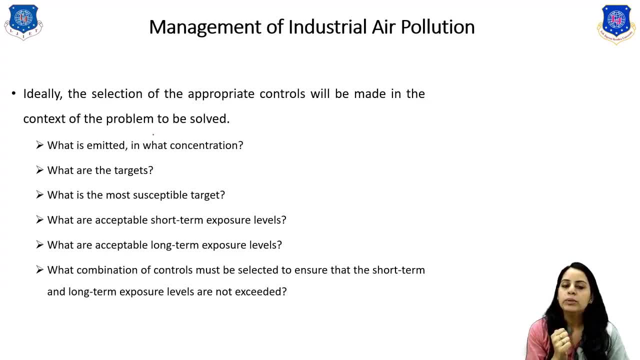 side control will be made in the context of the problem to be solved. first of all, what is emitted in what concentration and what are the targets? what are the most susceptible target then? what are the acceptable short-term exposure levels then? what are the acceptable long-term exposure levels? 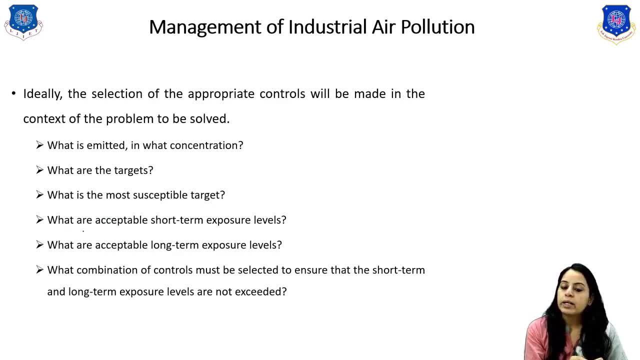 then what combination of control must be selected to ensure that the short-term and long-term exposure level are not exceeded? okay, so these all are the some question which is coming comes in our mind by the uh at the management level right now. the next one, which is the steps in selecting for the cell. 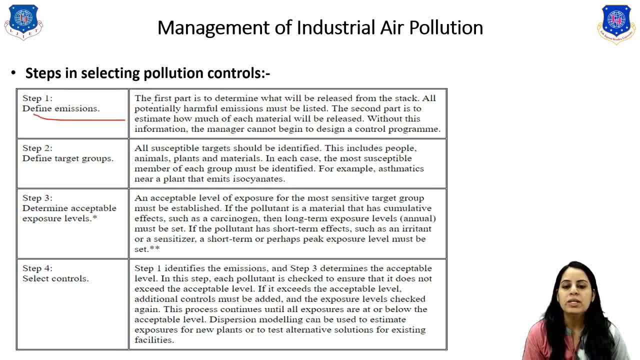 control. the first one, which is the defined ambition. it means that this is the first part, to determine what will be released from this time. okay, all the potentially harmful ambition must be listed. the second part is to eliminate how much of each material will be reduced. so, without this, 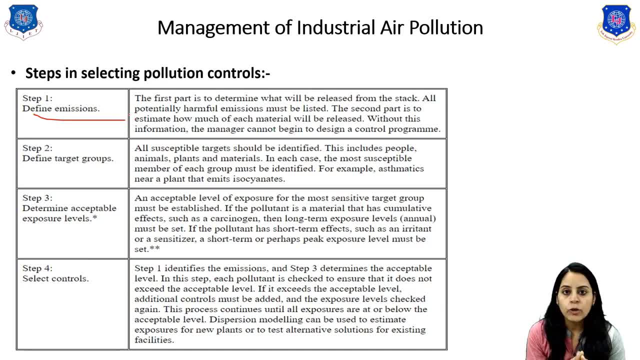 information, the manager cannot begin the designer control program right. okay, now the second step, which is the define the target group. it means the target group, which is the target group, which is the hatter. all susceptible targets should be identified after that. this includes the people, animal, plant and material. in each case, the most acceptable member of each group must be identified. 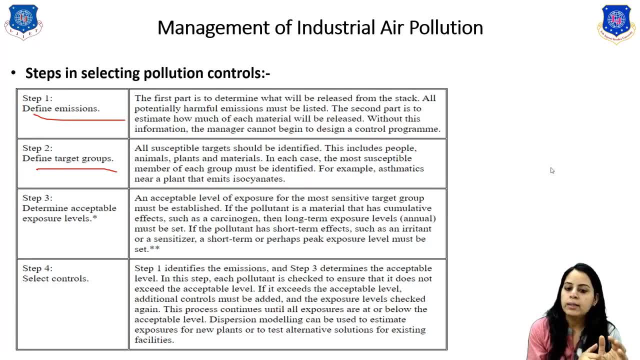 for example, asthmatics near a plant that added up isodine right. there is step three, which is determine the acceptable exposure level. means that the acceptable level of the exposure for the most sensitive target group must be established. if the pollutant is a material that has cumulative effect, such as the carcigin, then long-term exposure level. 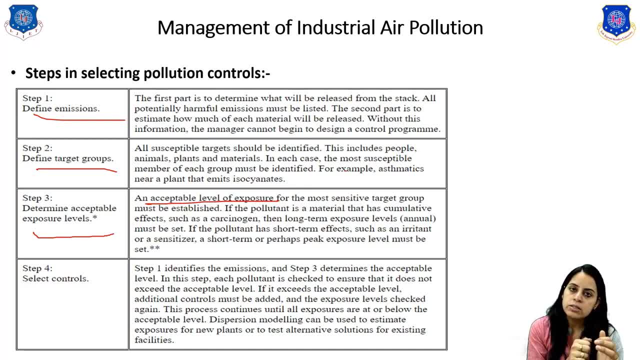 annual must be set okay, so that if pollutant has a soft term effect, such as the irritant or a sensitizer, or short term, perhaps a peak exposure level wants to be set okay. so this means that if the pollutant is a material that has cumulative effect, such as the irritant or a sensitizer, 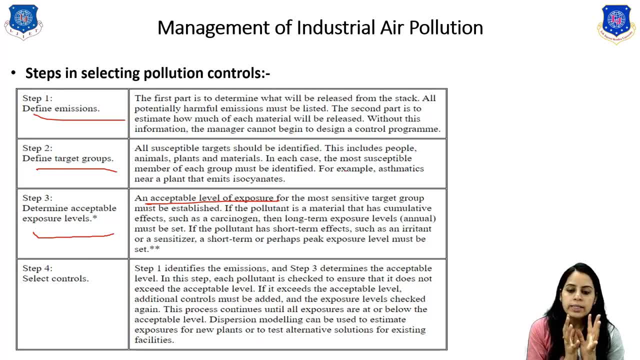 then the level of the exposure level must be set, okay. and the step four, which is select the control technique. okay. so the in step one, identify the emissions. first we identify the emission. and the step three, we determine the acceptable level. okay, so in this step, each pollutant is. 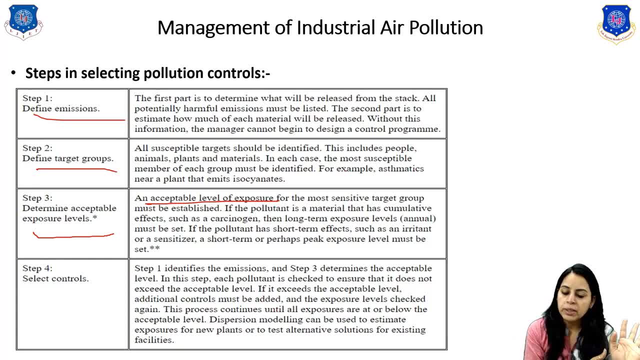 checked to ensure that it does not exceed the acceptable level. and if we exceed the acceptable level, then it must be needed. okay, so the exposure level check again. this process continue until all the exposure are at or below the acceptable level. right, so the dispersion modeling can be. 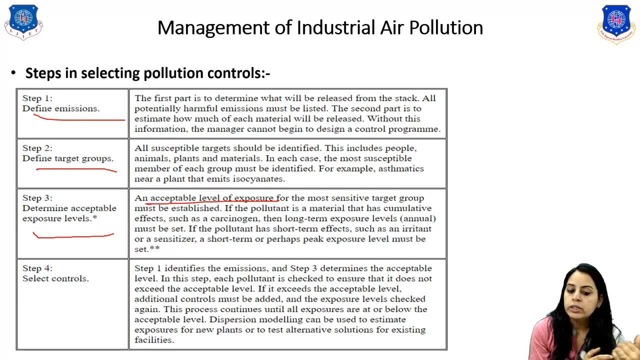 used to estimate the exposure for a new plant or a taste alternative solution for existing facilities. right? so this is the various steps in selecting the pollution control, the first one which we define. first of all, we define the application, right. uh, it means that to determine what will be. 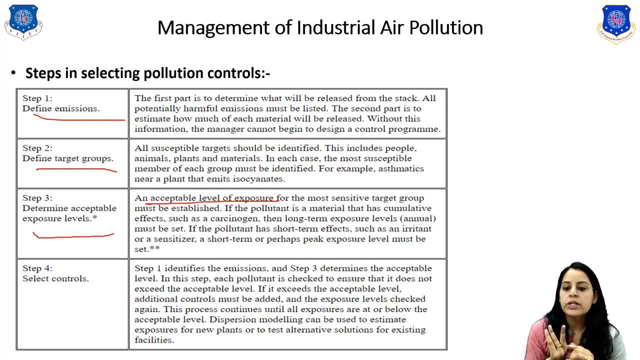 released from this time. okay, then the second one, which is the define the target group. it means that, first of all, it will be target, should be the identity point, right? okay, then step three. it means that determine the acceptable exposure level. it means that it is a less, a lace exposure level. 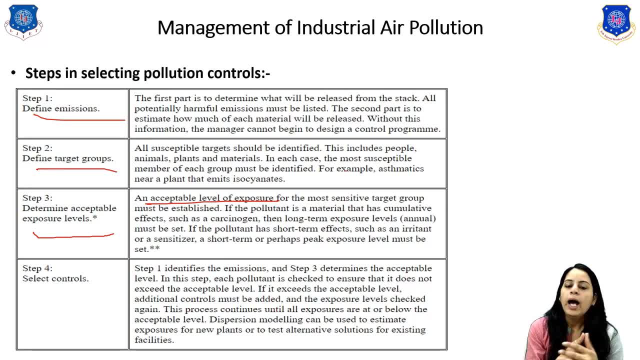 than a short term or long term exposure level right. and then the second one, which is the last four, which is the select, the control right. for example, if we identify the emission, then determine the accepted level, so in the search that in such a time the pollutant is checked. 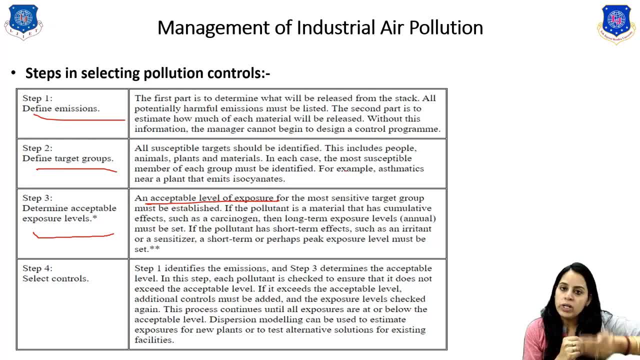 we saw that it is not exactly acceptance level. if they are exceeded for acceptance level, then we select the, select the another control for this particular pollutant. okay, so this is the scraps in selecting the pollution control, right? so this is all about the today's lecture. in today's lecture we discussed the various, the manage or industrial air pollution management. 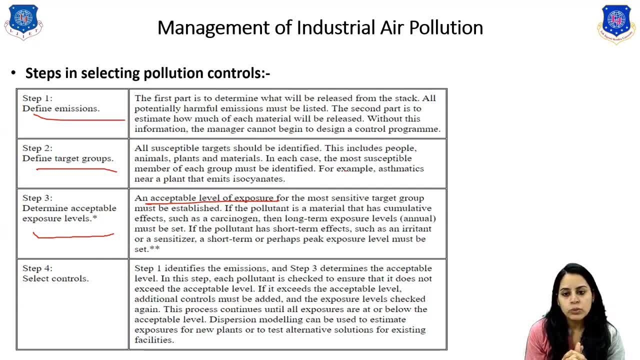 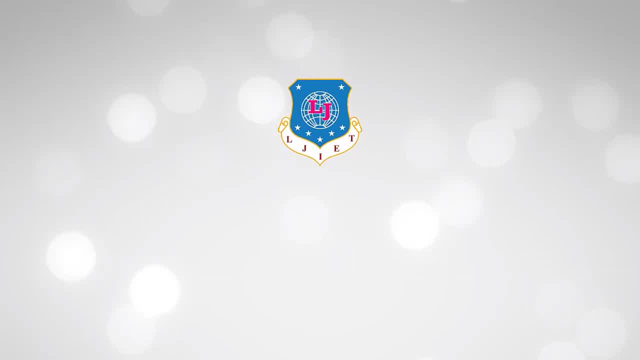 system right. i hope you all understood about the today's lecture. thank you for the watching. thank you.